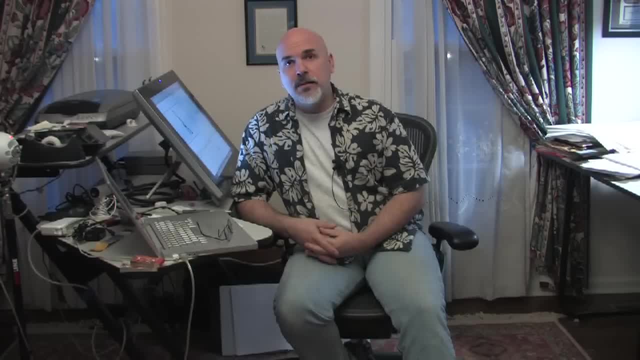 pastel on paper or markers- There are so many different media you can use And remember. for each minute of film it's 1,440 drawings. So you've got to mind for a five or six minute cartoon, you're talking close to 10,000 different images that you're going to be creating. If you're going to have voices in your cartoon, record them first, because you want to give your actors the freedom to. 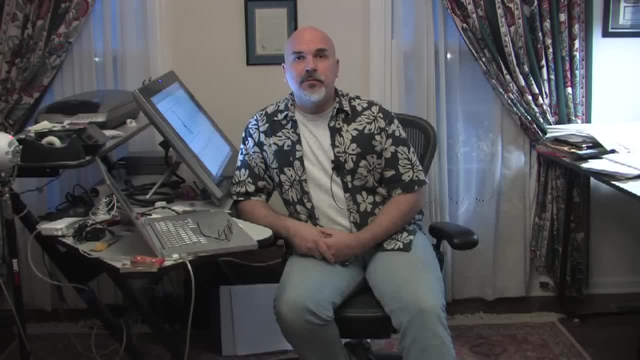 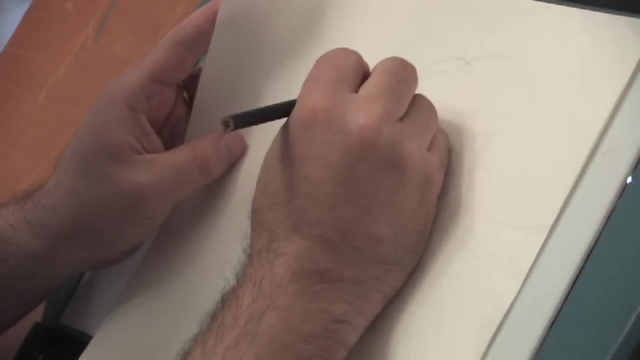 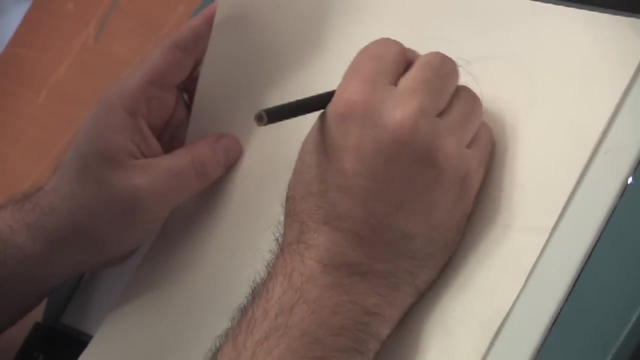 act and to ad-lib and to come up with funnier lines than maybe the ones you wrote, And that way you animate your character to the performance that's already been given. This is an animation disc And you can see how there are pegs and holes to hold your paper still, And that way you know each drawing is in the same place and it doesn't shake all around when you go to film it. 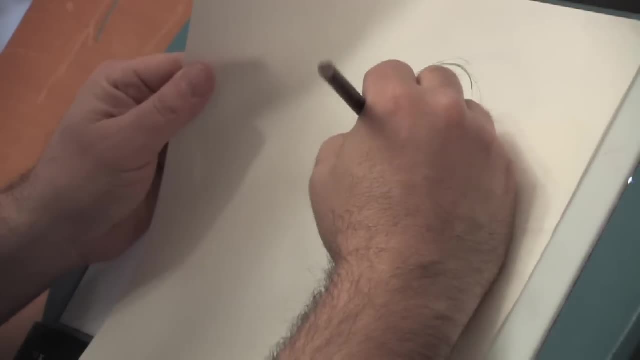 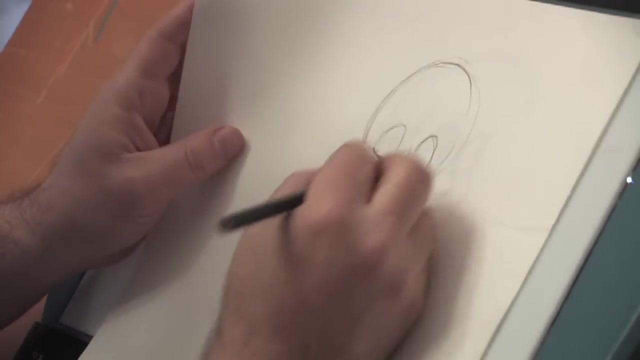 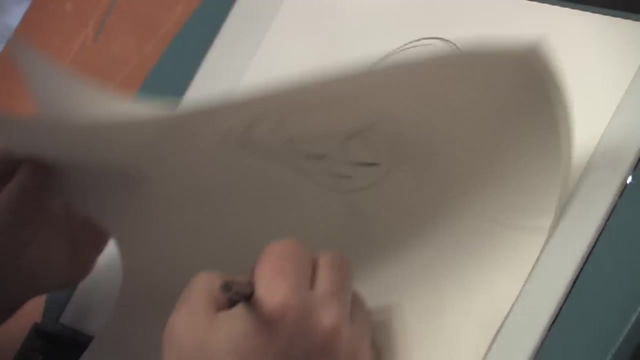 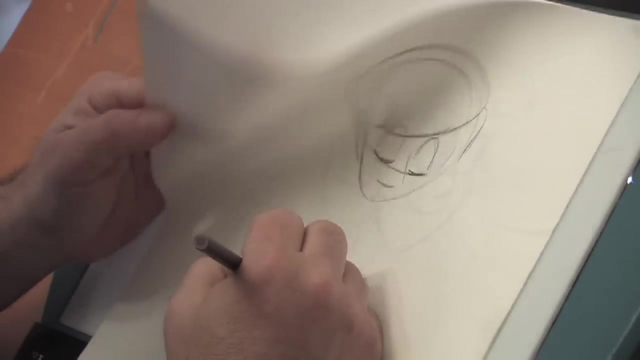 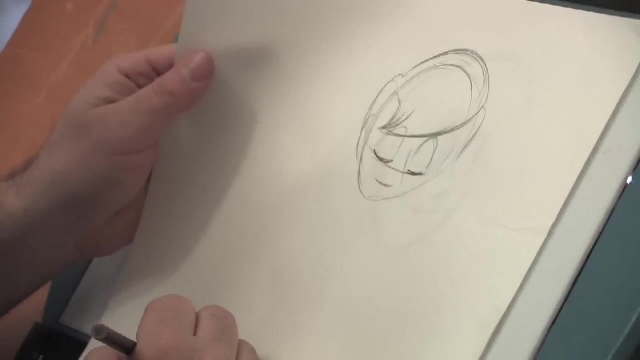 And you can buy specially punched paper that's got matching holes in it, And you can buy specially punched paper that's got matching holes in it. You can see, this is called in-betweening. when I'm doing my drawing one and this is the. 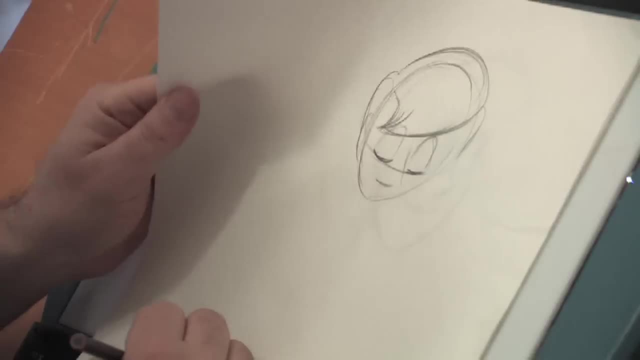 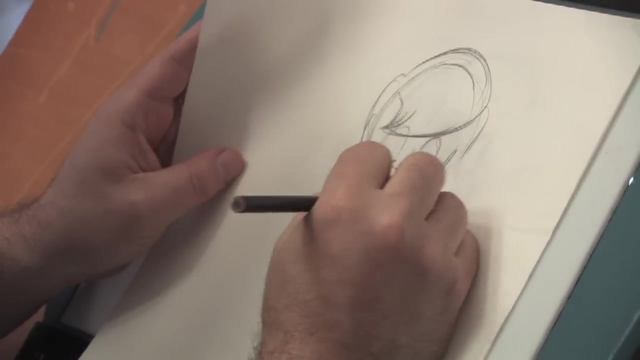 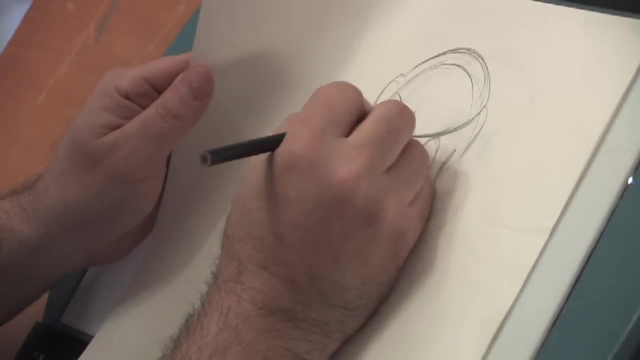 middle drawing and this is the drawing at the end. So I flip them back and forth and I can watch this kid's head turn And notice how his hair it kind of remains. it's still going this direction while he turns his head. 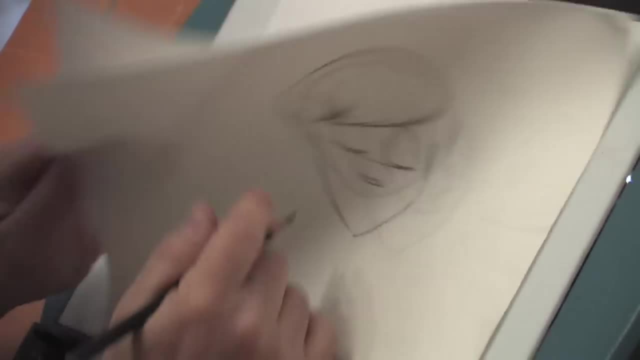 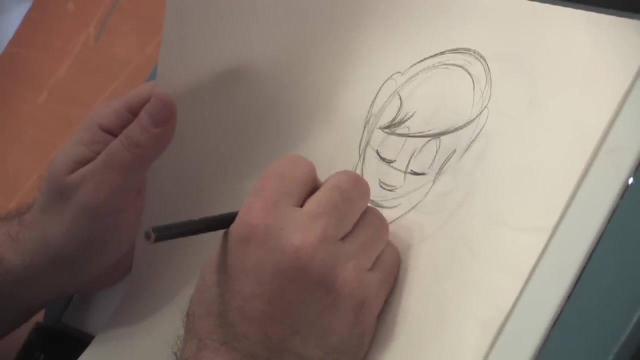 That's called drag. When something moves, it doesn't always go there at the same time, Like when a flag is blowing and you're waving it around. the part that doesn't move as fast is called drag, And the looser the object is, the more drag it will have.